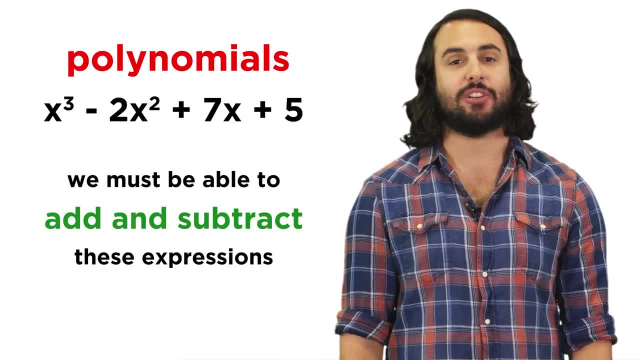 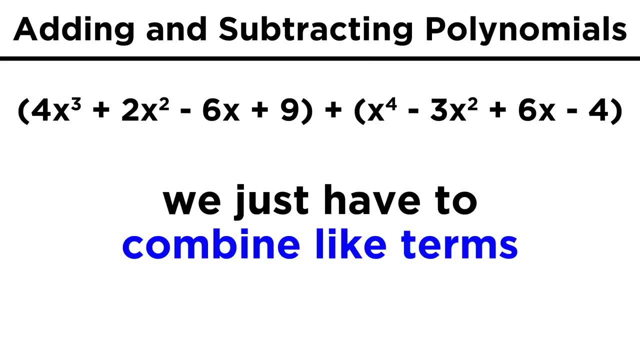 operations. Let's start with the simplest operations: addition and subtraction. When we add and subtract polynomials, the key is to combine like terms, because we want a single x to the fourth term, a single x cubed term, and so on. 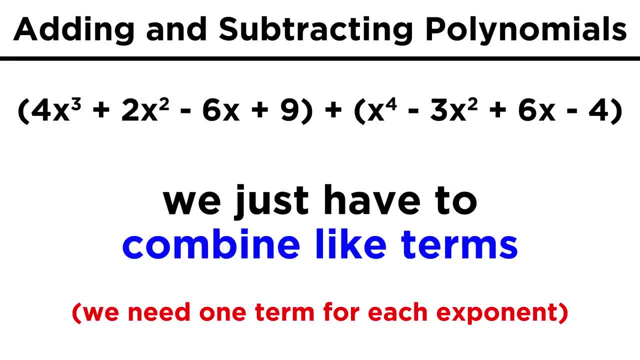 For any exponents that happen to be present in the expressions When we combine like terms. this is the same application of the distributive property that we have already learned, Just as five x plus four x is equal to the quantity of five plus four times x or nine. 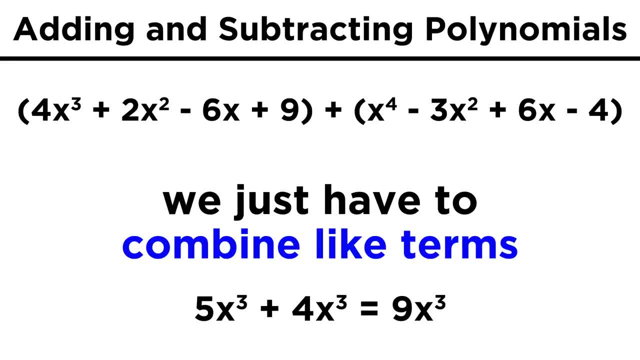 x. this will apply to five x cubed plus four x cubed. We can ignore the exponent for a moment, because we can simply recognize that they match. If they match, it doesn't matter what the term is, We will only manipulate the coefficient. 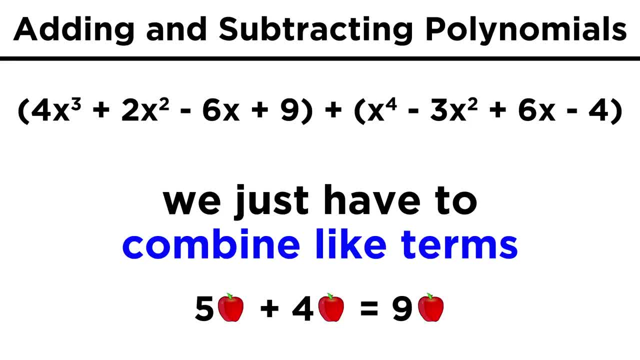 Five x cubed plus four x cubed may as well be five apples plus four apples, where the symbol of the apple can be taken to represent x cubed. Once we see things that way, it is easy to see how these terms add together to become: 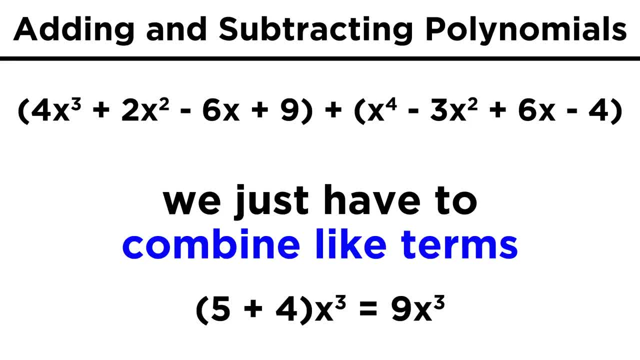 nine x cubed. This is also apparent when we apply the distributive property, as x cubed could operate across the sum of five plus four. Now let's add two x's. If we add two whole expressions together, four x cubed plus two x squared minus six. 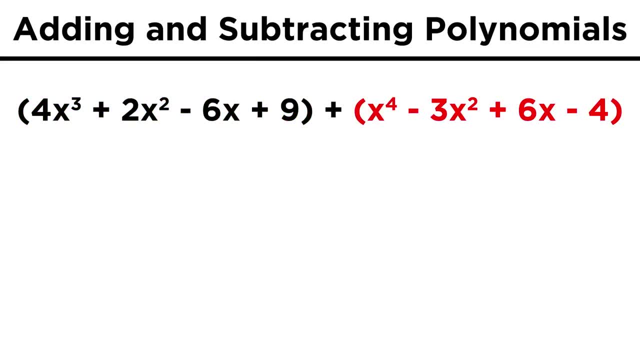 x plus nine will be one expression, and the other is x to the fourth minus three, x squared plus six, x minus four. If we want to add these together, there are several ways we could do it, and whichever way works best for you is just fine. 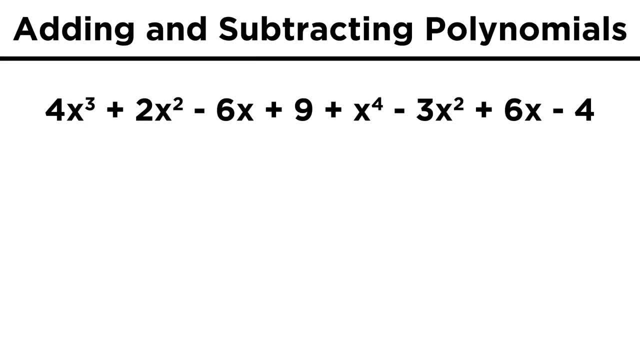 We could just write a new expression with all of these terms in a line if we wanted. Then it's just a matter of identifying like terms. However, a slightly tidier approach, if you value that sort of thing, could involve putting one expression over the other so that we can do arithmetic just the way we did with 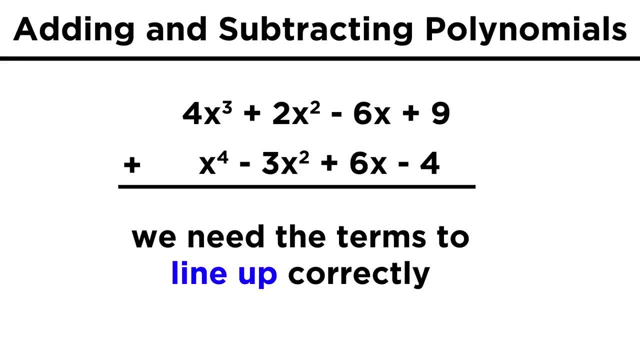 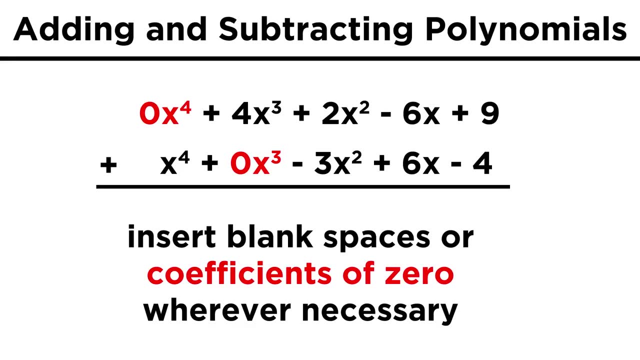 small numbers. If we do this, it is important to notice the degree on each term and make sure the exponents are lined up properly so that we add or subtract the correct terms. This could involve leaving a blank space if a particular exponent is not present in an 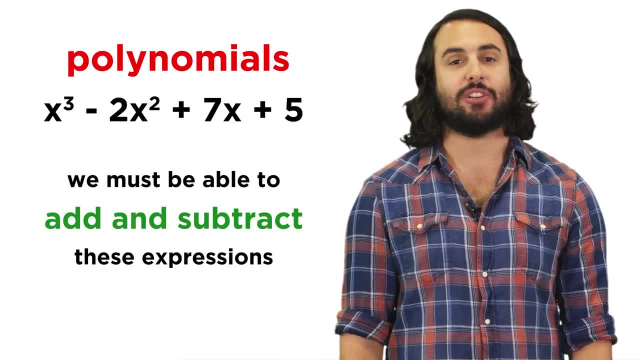 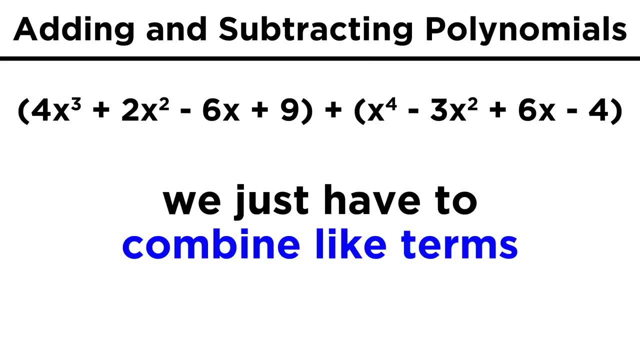 operations. Let's start with the simplest operations: addition and subtraction. When we add and subtract polynomials, the key is to combine like terms, because we want a single x to the fourth term, a single x cubed term, and so on. 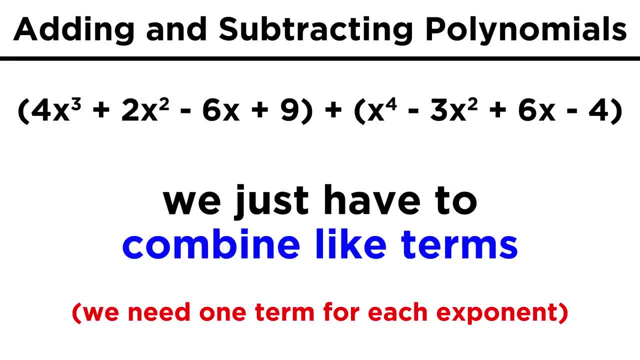 For any exponents that happen to be present in the expressions When we combine like terms. this is the same application of the distributive property that we have already learned, Just as five x plus four x is equal to the quantity of five plus four times x or nine. 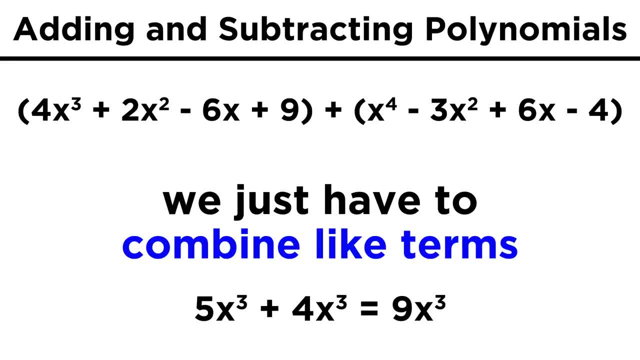 x. this will apply to five x cubed plus four x cubed. We can ignore the exponent for a moment, because we can simply recognize that they match. If they match, it doesn't matter what the term is, We will only manipulate the coefficient. 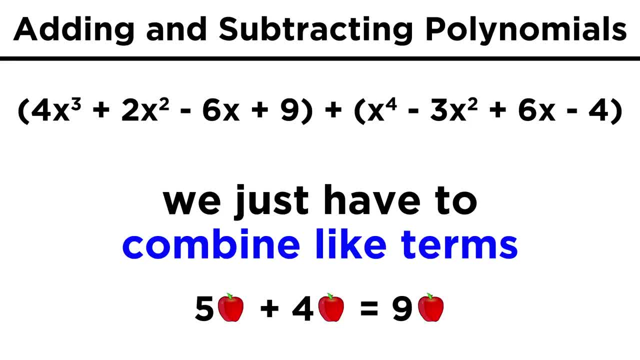 Five x cubed plus four x cubed may as well be five apples plus four apples, where the symbol of the apple can be taken to represent x cubed. Once we see things that way, it is easy to see how these terms add together to become: 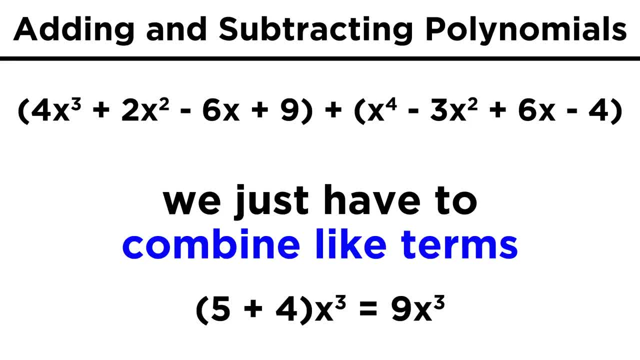 nine x cubed. This is also apparent when we apply the distributive property, as x cubed could operate across the sum of five plus four. Now let's add two x's. If we add two whole expressions together, four x cubed plus two x squared minus six. 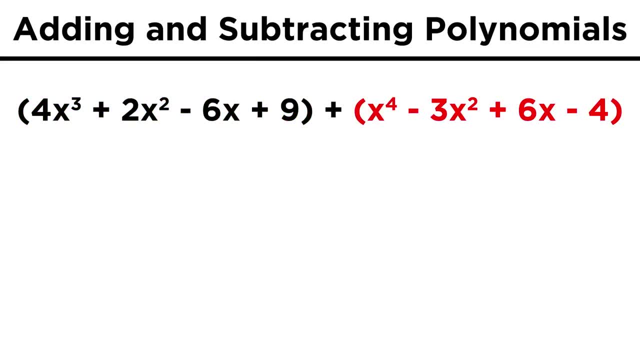 x plus nine will be one expression, and the other is x to the fourth minus three, x squared plus six, x minus four. If we want to add these together, there are several ways we could do it, and whichever way works best for you is just fine. 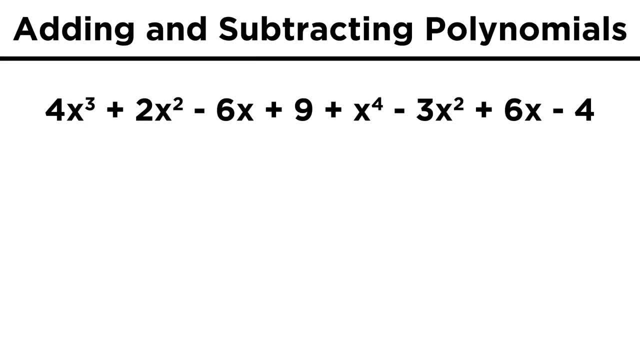 We could just write a new expression with all of these terms in a line if we wanted. Then it's just a matter of identifying like terms. However, a slightly tidier approach, if you value that sort of thing, could involve putting one expression over the other so that we can do arithmetic just the way we did with 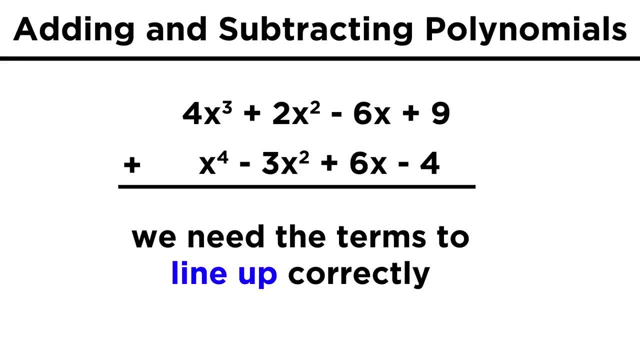 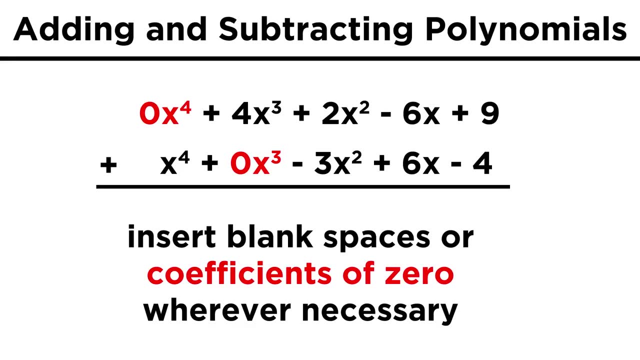 small numbers. If we do this, it is important to notice the degree on each term and make sure the exponents are lined up properly so that we add or subtract the correct terms. This could involve leaving a blank space if a particular exponent is not present in an 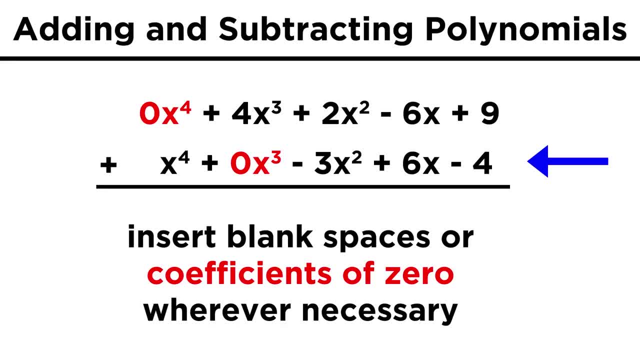 expression Like this one, which does not have an x cubed term. This kind of bookkeeping will help us avoid making a careless error. Now, with everything lined up, we just add X to. the fourth is by itself, so we leave it alone. 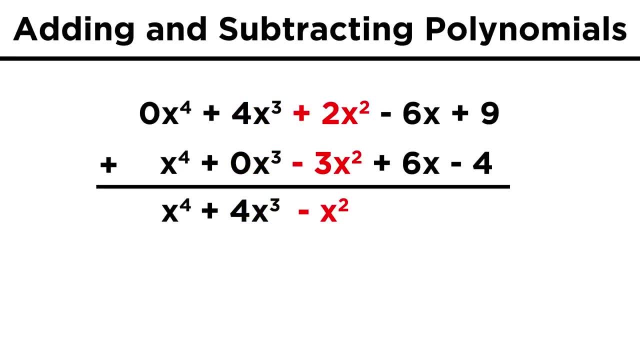 Same with four x cubed. that will stay as is. Then we have two x squared minus three x squared, which leaves us with negative x squared. Negative six x plus six x leaves us with zero for the x term, and nine minus four is five. 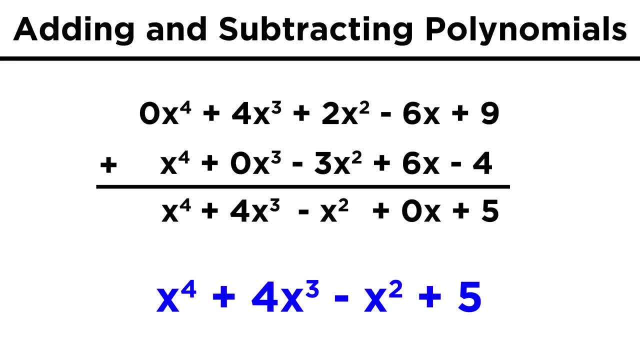 So x to the fourth plus four, x cubed, minus x squared plus five will be the answer. Subtraction is essentially the same, we just have to be a little more careful about our signs. Let's say, we keep each expression as it is, but we subtract the second one from the 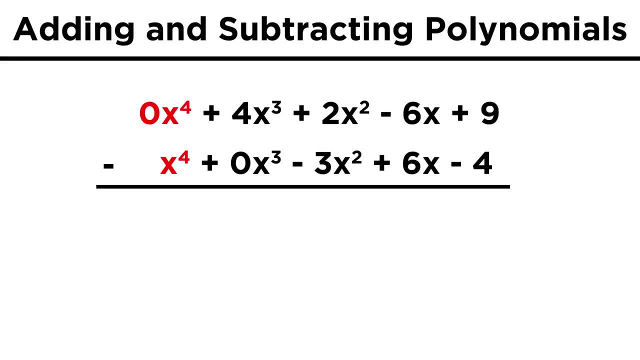 first one. Now we are subtracting x to the fourth from zero x to the fourth. That gives negative x to the fourth. Then it's four x cubed minus zero, so that term stays as it is. Then it's two x squared minus negative three x squared. 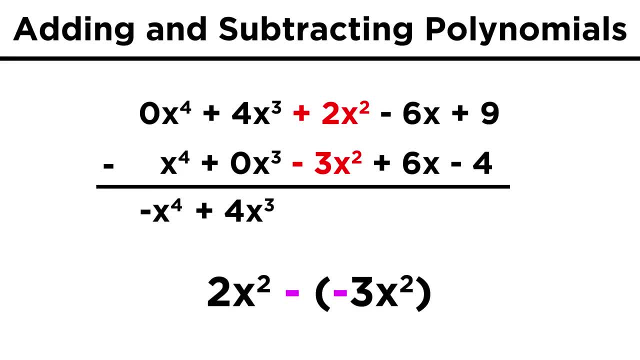 Remember that subtracting a negative number is the same as adding the positive version, So this becomes two x squared plus three x squared or five x squared Negative. six x minus six x is negative twelve x and nine minus negative four is thirteen. 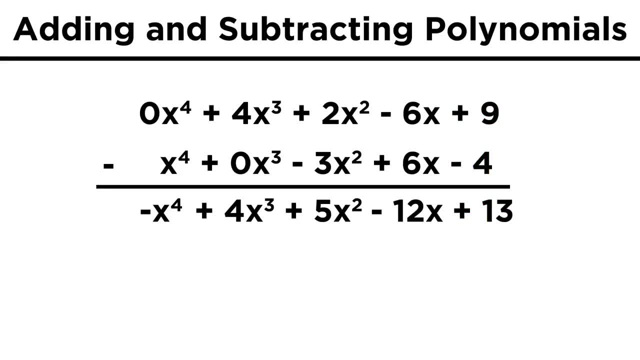 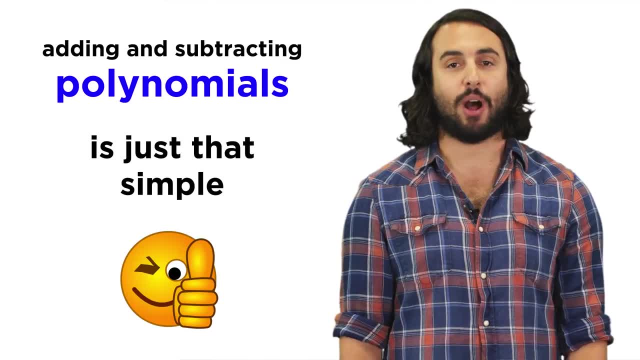 And this is how we subtract one polynomial from another. So that's all there is to it for the addition and subtraction of polynomials. Things get trickier when we subtract one polynomial from another. So let's take a look. It's even trickier when we try to multiply polynomials. 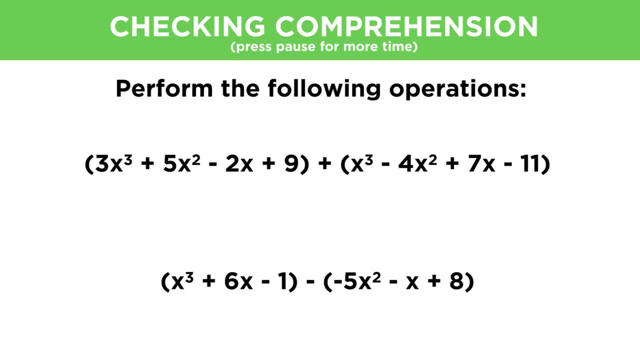 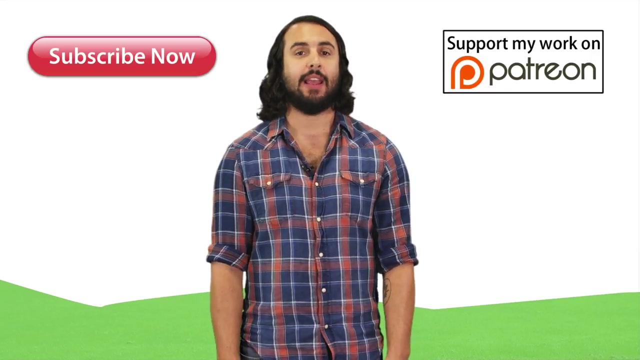 But before we move on to that, let's check comprehension. Let's take a look. Thanks for watching, guys. Subscribe to my channel for more tutorials. Support me on Patreon so I can keep making content And, as always, feel free to email me professordaveexplains at gmail dot com. 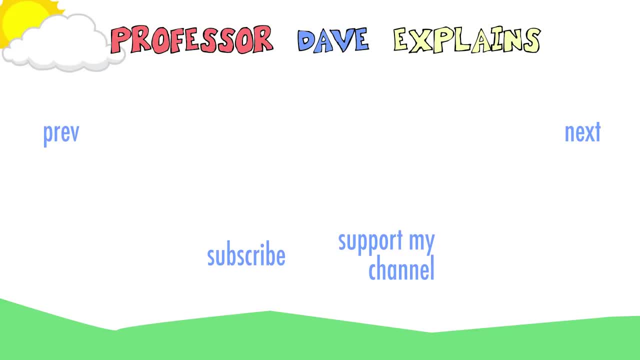 I'll see you in the next one. Bye. 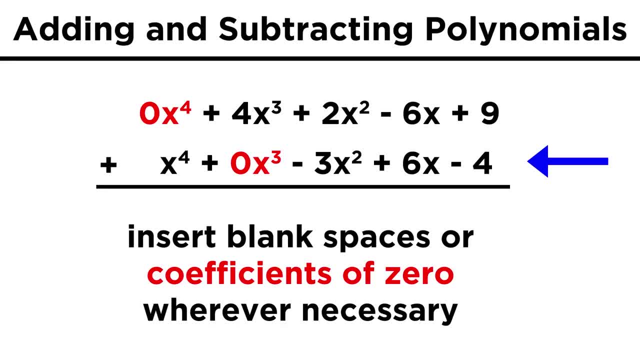 expression Like this one, which does not have an x cubed term. This kind of bookkeeping will help us avoid making a careless error. Now, with everything lined up, we just add X to. the fourth is by itself, so we leave it alone. 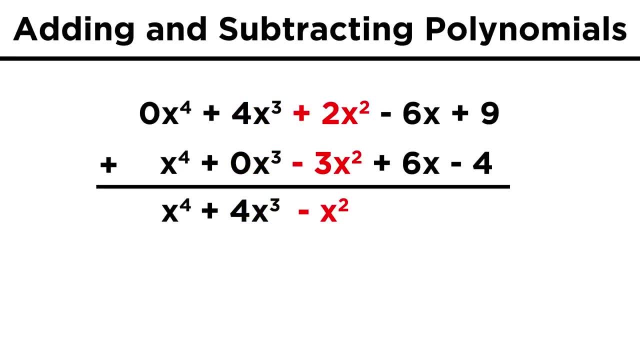 Same with four x cubed. that will stay as is. Then we have two x squared minus three x squared, which leaves us with negative x squared. Negative six x plus six x leaves us with zero for the x term, and nine minus four is five. 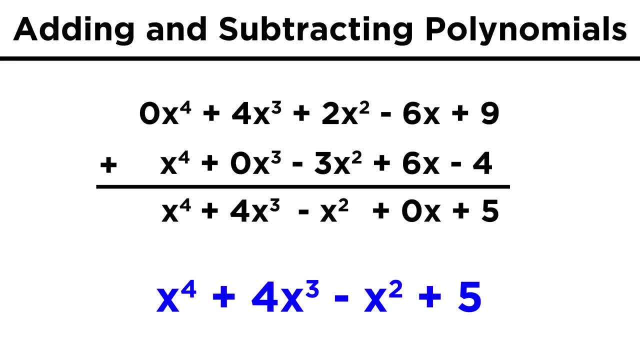 So x to the fourth plus four, x cubed, minus x squared plus five will be the answer. Subtraction is essentially the same, we just have to be a little more careful about our signs. Let's say, we keep each expression as it is, but we subtract the second one from the 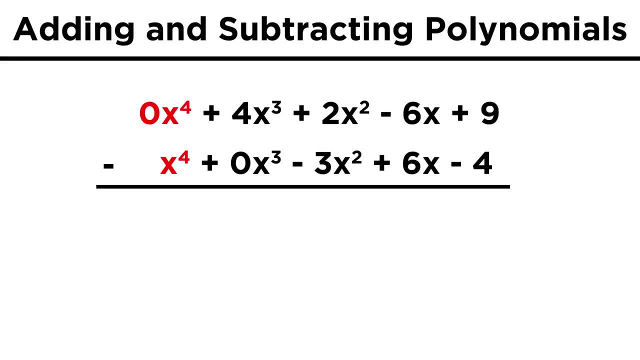 first one. Now we are subtracting x to the fourth from zero x to the fourth. That gives negative x to the fourth. Then it's four x cubed minus zero, so that term stays as it is. Then it's two x squared minus negative three x squared. 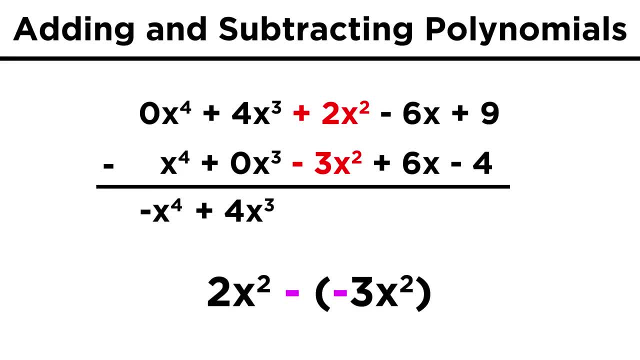 Remember that subtracting a negative number is the same as adding the positive version, So this becomes two x squared plus three x squared or five x squared Negative. six x minus six x is negative twelve x and nine minus negative four is thirteen. 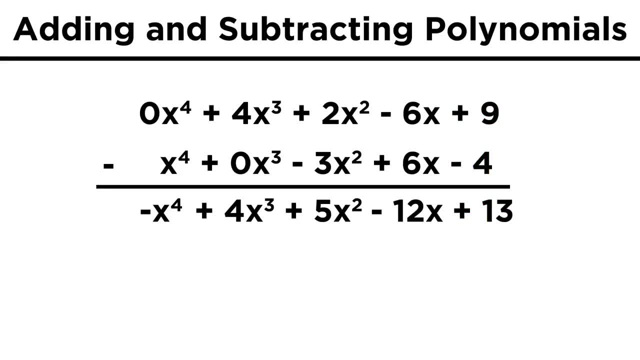 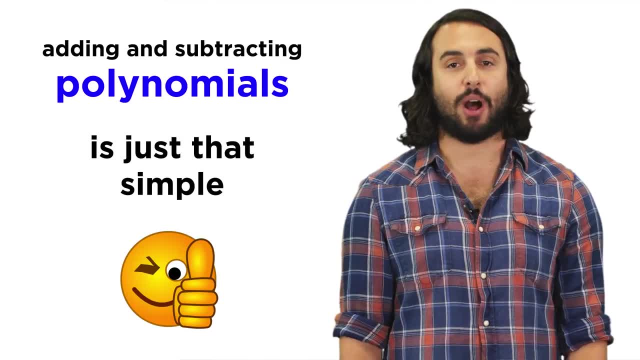 And this is how we subtract one polynomial from another. So that's all there is to it for the addition and subtraction of polynomials. Things get trickier when we subtract one polynomial from another. Things get trickier when we try to multiply polynomials. 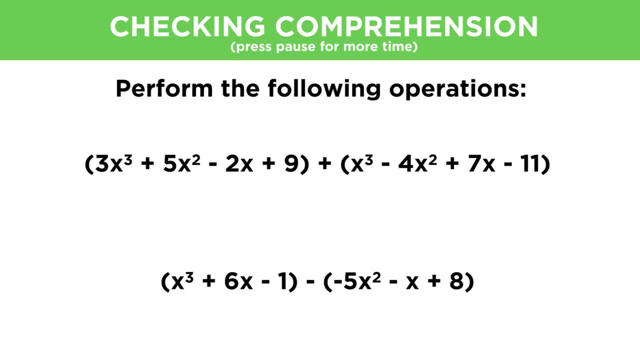 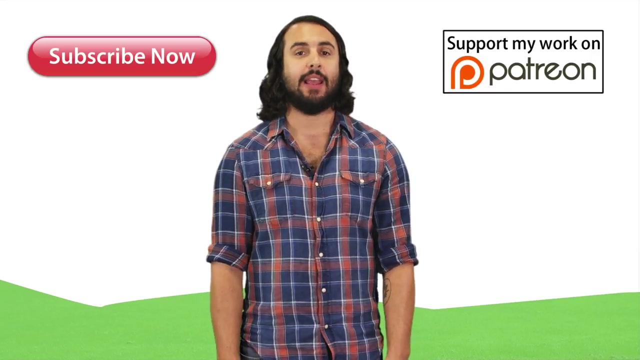 But before we move on to that, let's check comprehension. Thanks for watching, guys. Subscribe to my channel for more tutorials. Support me on Patreon so I can keep making content And, as always, feel free to email me professordaveexplains at gmail dot com. 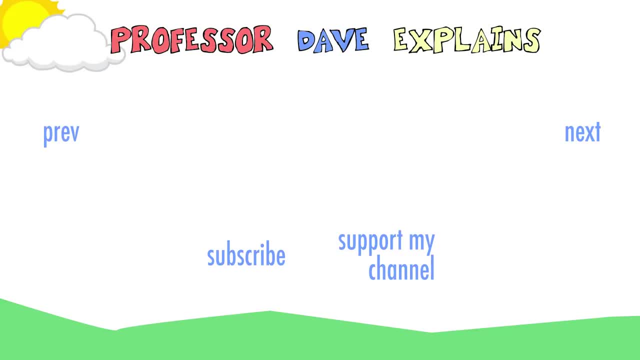 I'll see you next time. Bye-bye.